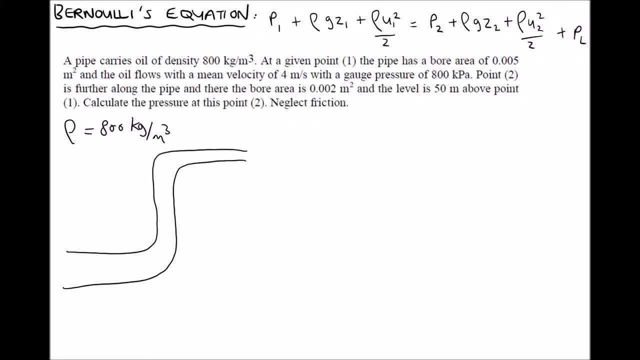 just a rough sketch. We know that 0.2 is 50 m above 0.1.. So if we add a dashed line to our centre line, Then we know that this distance here is 50 m. We have a change in elevation. The question: 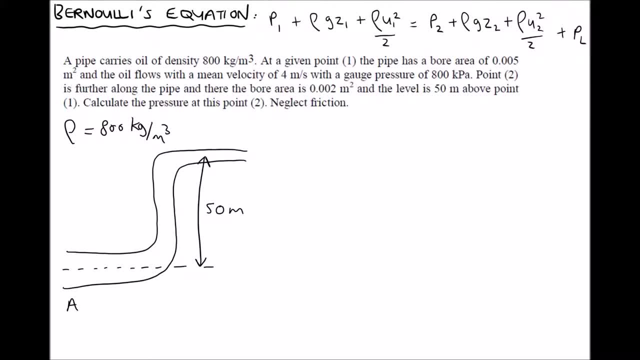 also told us that at position 1, the area- so A1, was 0.005 m2.. That's already in SI units And it has a mean velocity, u1, at that point, of 4 m per second. We're also given the pressure at position 1, of 800 kPa. 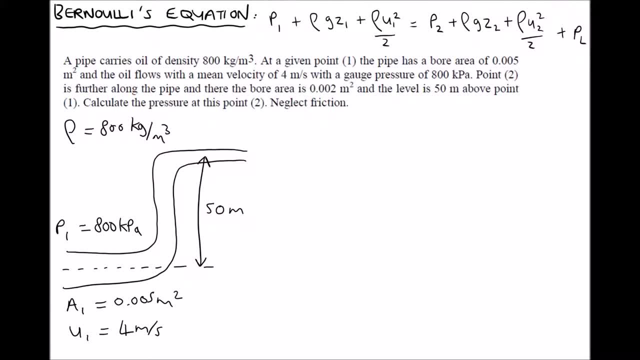 It gives us some information about position 2.. It tells us that the area at position 2 is 0.002 m2. But it doesn't give us any further information. It doesn't tell us the pressure at point 2, because that's what it wants us to calculate. 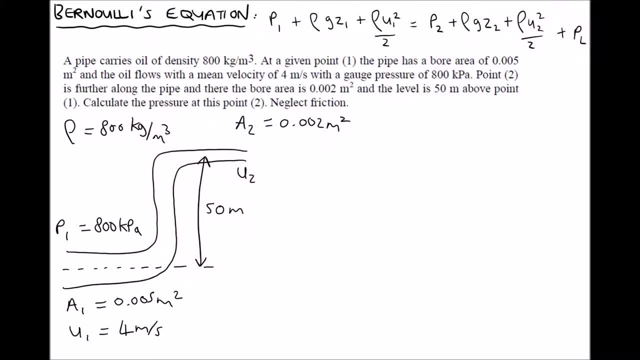 calculate, and it doesn't tell us the velocity at point two, But we're going to need to determine the velocity at point two in order to calculate the pressure at point two. The other thing that it tells us is that we can neglect friction. It tells us that right at the end of the question. 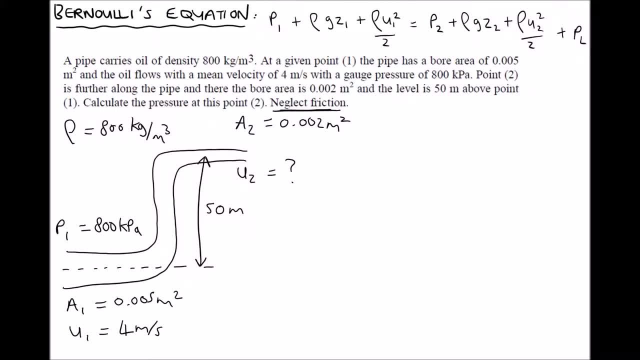 there. So first of all, then, let's see what terms we can get rid of. We have the Bernoulli's equation at the top, moving from left to right, P1, but we have a value of P1 given, so we 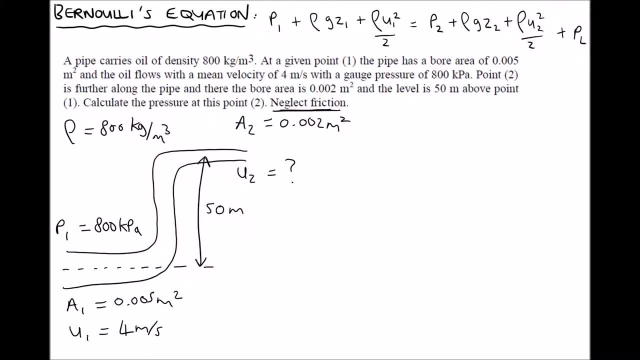 can't lose that term. Next, we have the term rho GZ1.. Well, if we use position one as our datum, then the elevation of position one is zero. The elevation of position two relative to position one is 50 meters. so it makes sense to set Z1 to zero, so we can get rid. 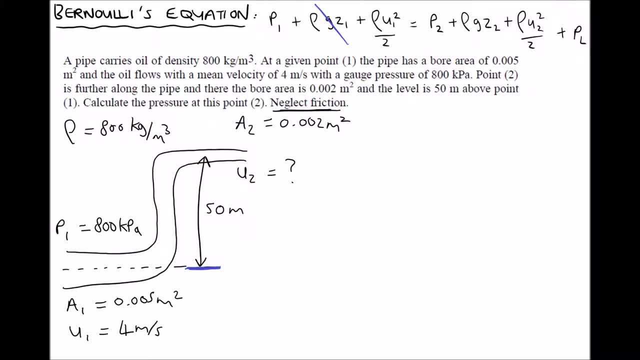 of that term. We then have rho U1 squared over two and we have a value given for U1.. Moving on, Moving to the right hand side, the question wants us to calculate P2, so we need to keep that term in. We have rho GZ2, well, we have an elevation at position two relative to position. 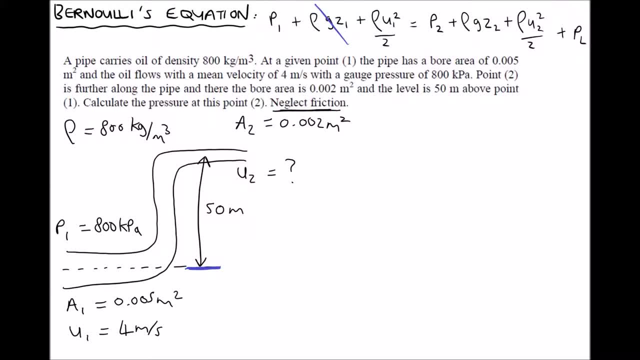 one, so we need to leave that term in. And we have rho U2 squared over two. well, we have a velocity at position two, so we need to leave that term in. It does tell us that we can neglect losses, so we'll lose PL. 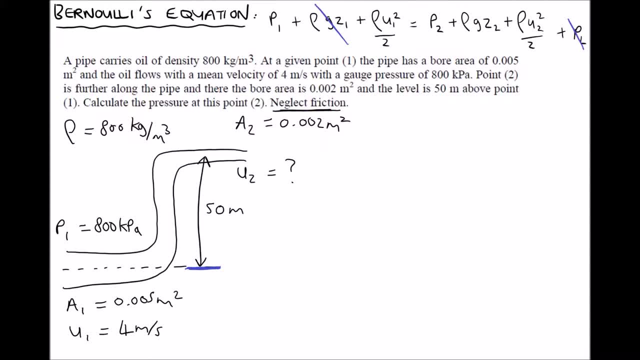 So one of the first steps here is to calculate U2.. We need to calculate U2 before we can calculate P2.. And we can use the continuity equation for this, because we know that U1- A1 equals U2- A2.. Now, from our question, we were given 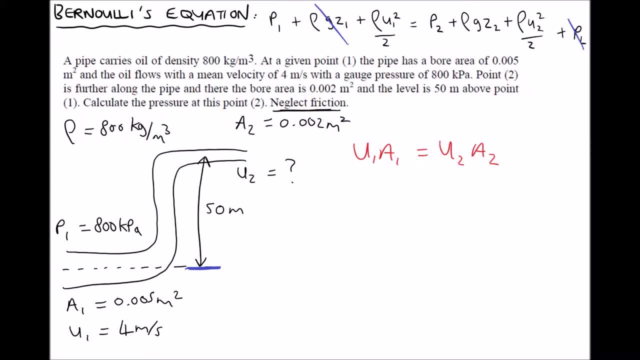 values for A1 and A2, and we were given a value for U1.. So let's rearrange this formula to make U2 the subject And to get U2 on its own, all we need to do is divide it by P2.. So we have rho, GZ1 squared over two. well, we have rho. 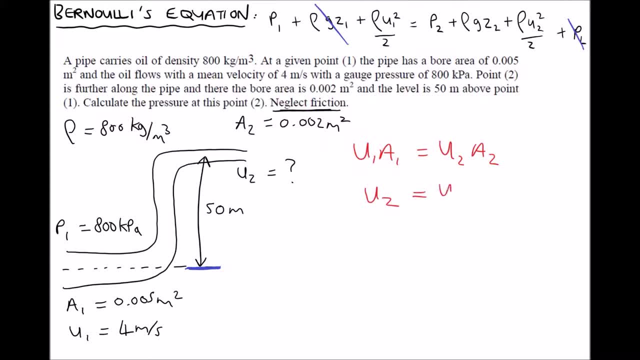 GZ1 squared over two, so we need to divide each side by A2.. So U2 is U1, A1 divided by A2. And plugging in values we get U2 equals four for U1, 0.005. 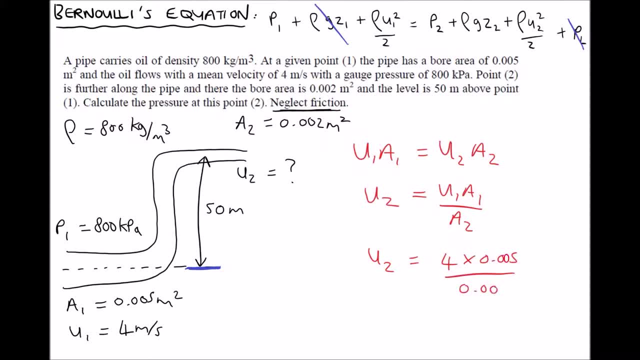 for A1, and 0.002 for A2,, giving us a value of U2 equal to 0.005.. So we've got a value of U2 equal to 10 meters per second. So let's add that value to our diagram and then we can calculate the pressure at position. 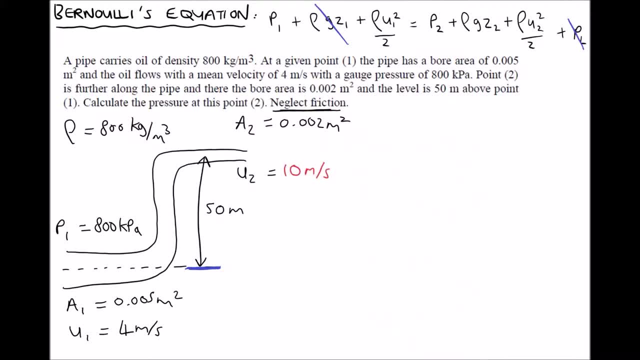 two. Okay, so we've been able to reduce our Bernoulli's equation by cancelling out a couple of terms. So our Bernoulli's equation is now just P1 plus rho- U1, squared over two, plus rho- GZ1 squared over two. 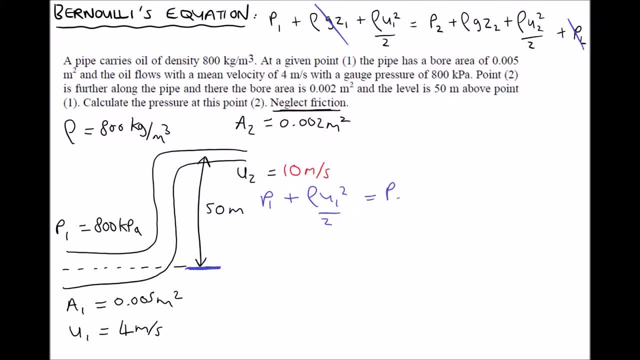 And then we can calculate the pressure at position two. Okay, so we've been able to reduce our Bernoulli's equation by cancelling out a couple of terms. So we've got a value of U2 equals P2 plus rho, GZ2 plus rho, U2 squared over two. 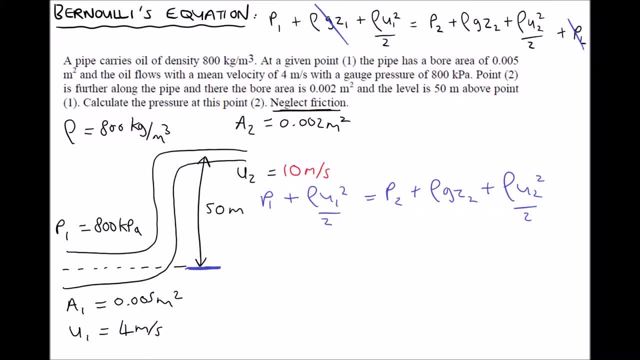 Now, the thing that we're trying to get on its own this time is P2.. So we need to subtract two terms from the right-hand side. We need to subtract rho GZ2, and we need to subtract rho U2 squared over two. 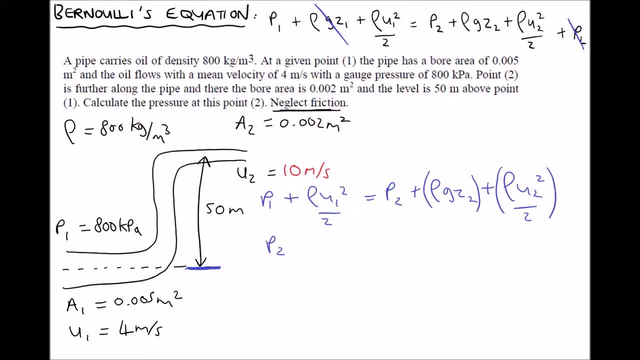 So we can rewrite this. We'll get P2 equals P1 plus rho U1 squared over two, minus rho GZ2, because we're subtracting that from the right-hand side- minus rho U2 squared over two, again because we're subtracting. 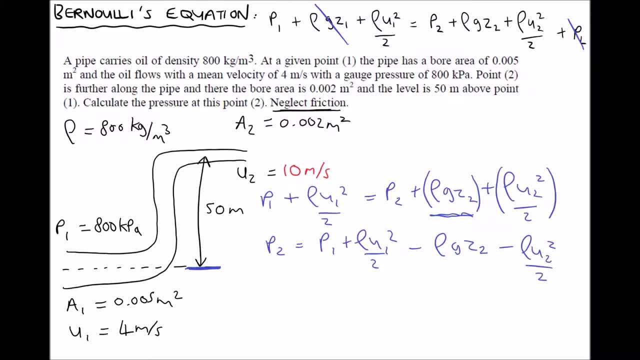 that from the right-hand side. Now it's just a case of plugging in our numbers, Because the pressure at position two is P1,. well, P1 is 800 kilopascals, or 800,000, plus rho U1 squared over two, well, we have our density, 800.. 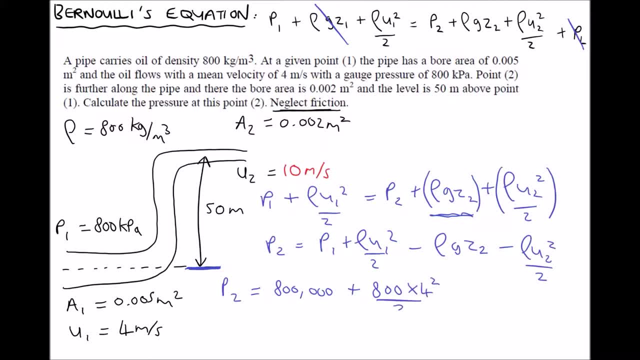 We have U1 as four. We have rho GZ2, so minus 800.. We have rho GZ2, so minus 800.. We have rho GZ2, so minus 800.. And now we're going to subtract rho GZ2, times gravity 9.81, times Z2, which is 50. 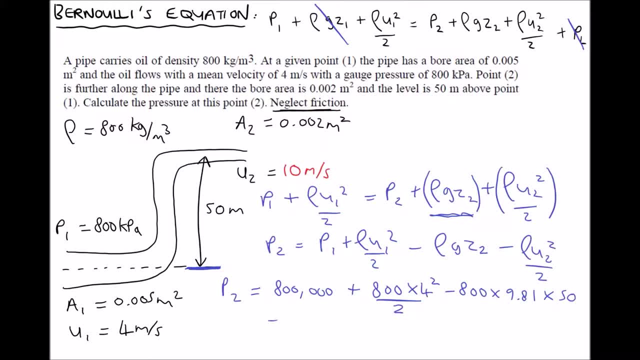 metres. And then we need to minus rho U2 squared over two, So 800.. U2, we said was 10 over two. So note that we're subtracting rho GZ2, and we're subtracting rho U2 squared over two. 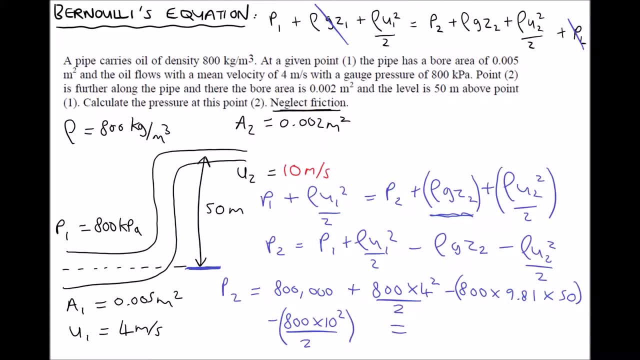 Now running that all through the calculator gives us a pressure at position 2 equal to 374,000 or expressed in kilopascals, 374 kilopascals. So from this example and the earlier example we've seen how we can take a descriptive question. 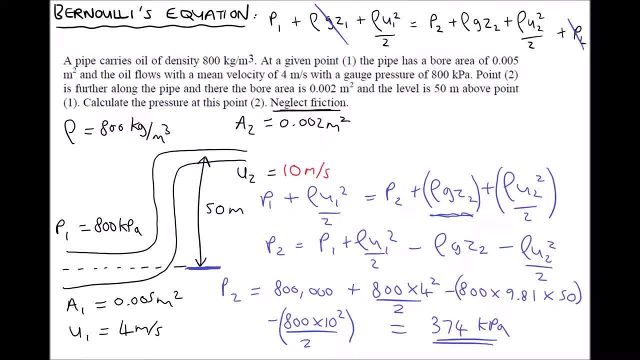 in order to produce a sketch of the scenario. and once we've produced a sketch of the scenario, we can refer back to our Bernoulli's equation and remove the terms that aren't relevant. Finally, we can determine the unknown parameters within the fluid system.